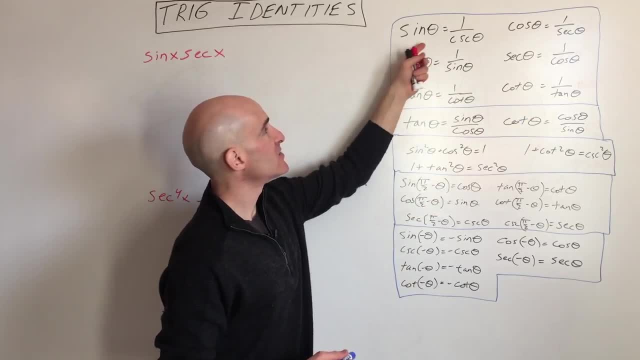 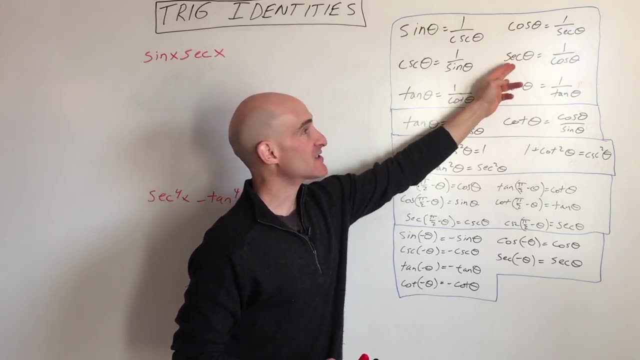 These are what are called the reciprocal identities, because you can see, like sine is the reciprocal of cosecant or cosecant is the reciprocal of sine, Cosine and secant are reciprocals of each other, Tangent and cotangent. So you can see how they're paired up with one. 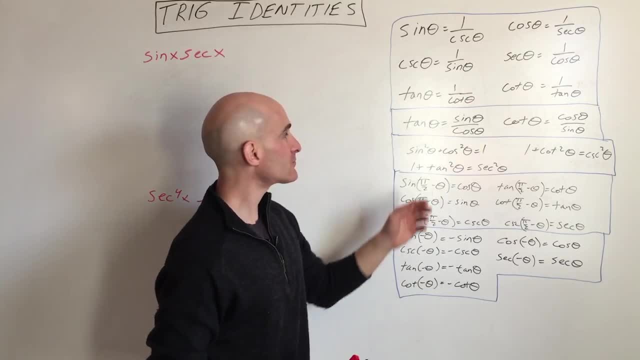 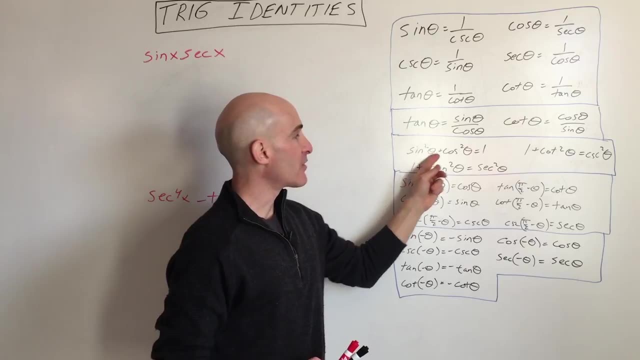 another, and that'll cut down on some of the memorization that you'll need to do. Tangent is sine over cosine, Cotangent is cosine over sine. And then we've got the three Pythagorean trig identities: Sine squared plus cosine squared equals one. And then to get these other two, what? 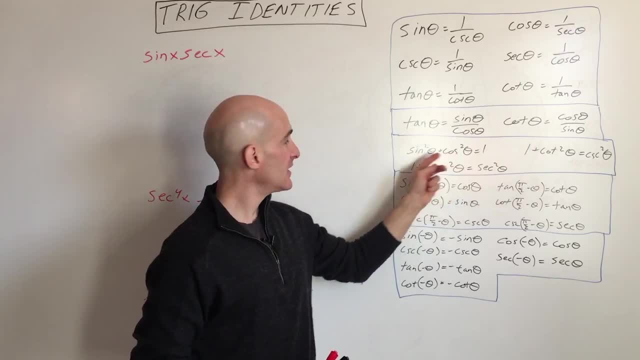 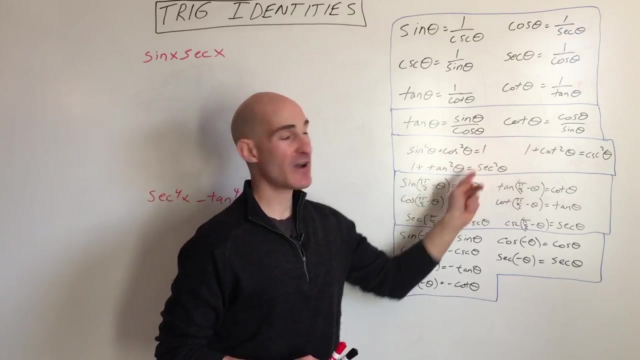 you can do is if you take the basic Pythagorean trig identity and you divide all of these quantities by sine squared, you'll get this one. And if you divide all these by cosine squared, you'll get this identity. So if you know this one, you'll be able to find these other two. 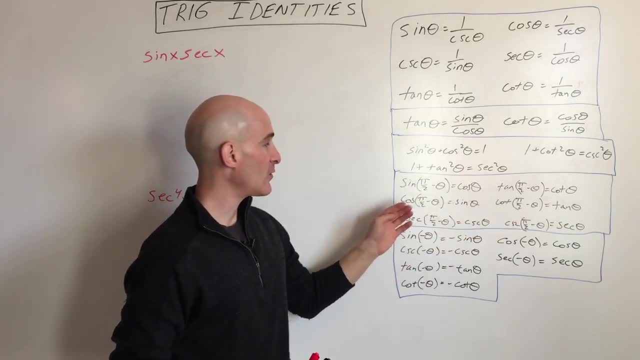 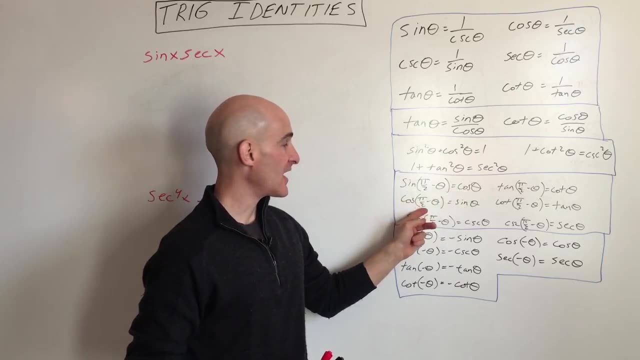 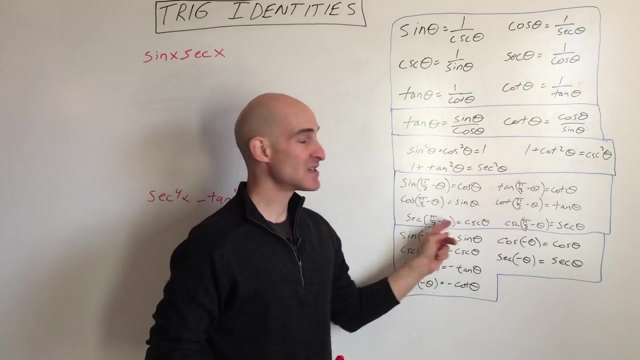 And then here what we have are the co-functions, And again what you can do is you can pair these up Like: sine of 90 minus the angle equals cosine. Cosine of 90 minus angle is sine. So sine and cosine are co-function pairs. Tangent and cotangent are co-function pairs, Secant and cosecant go. 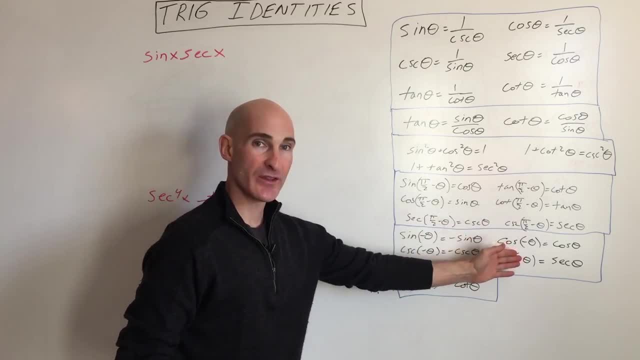 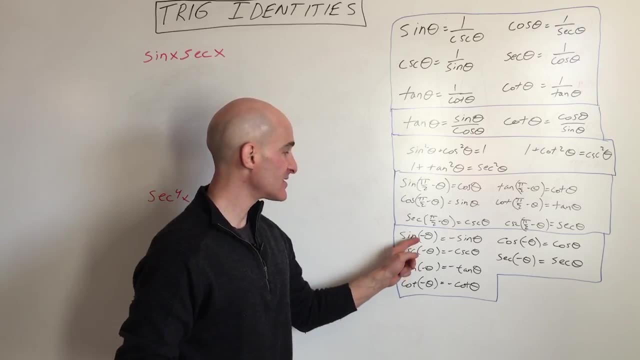 together. These ones here are what are called the even and odd identities, And what you'll notice here is that, sine cosecant, tangent and cotangent are odd, And what that means is that if you're taking the sine of a negative angle, it has the same value as the sine of a positive angle. 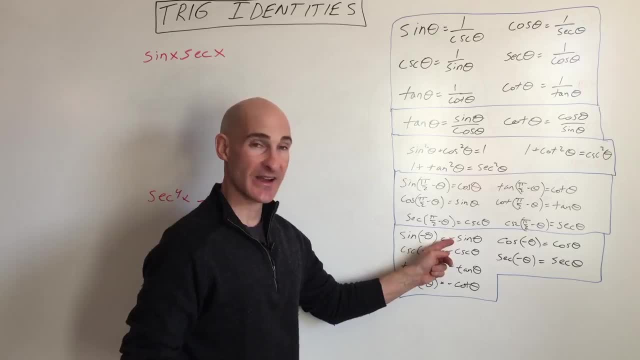 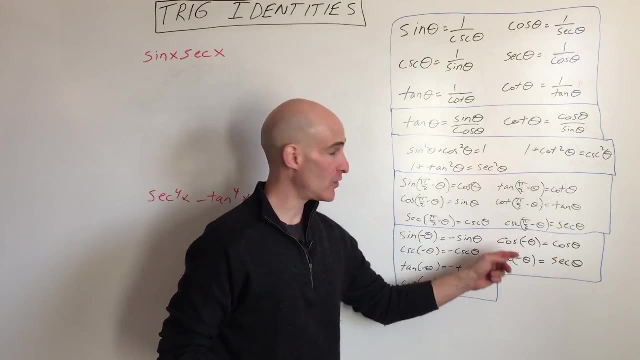 But it will have the opposite sign. So if this is negative, then be negative times. negative will be positive. So the signs will be the opposite. But cosine and secant, they're the same. So the cosine of a negative angle will be the same as the cosine of the positive angle. They'll be exactly. 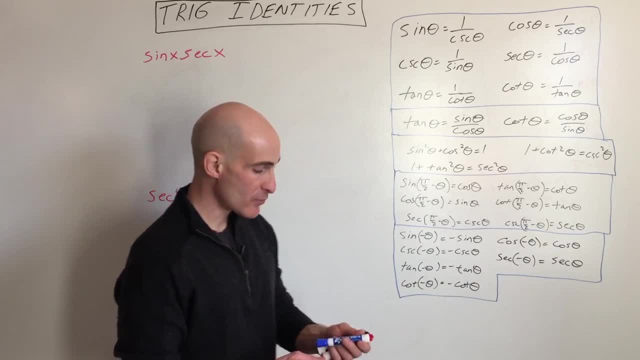 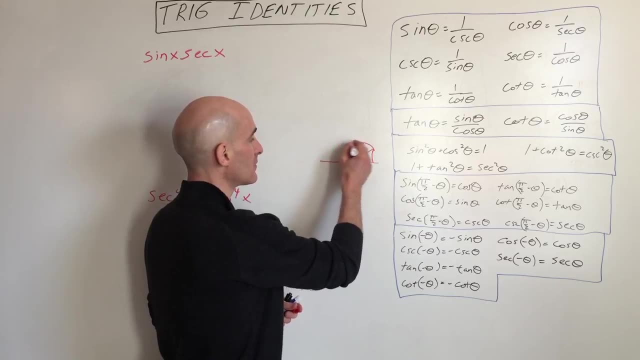 the same. And if you want to understand some of these a little bit deeper, I can show you a little bit more about it. Like say, for example, if you had a triangle like this: If you go this direction, that's positive. If you go this direction, that's negative. If you go this direction, that's negative. 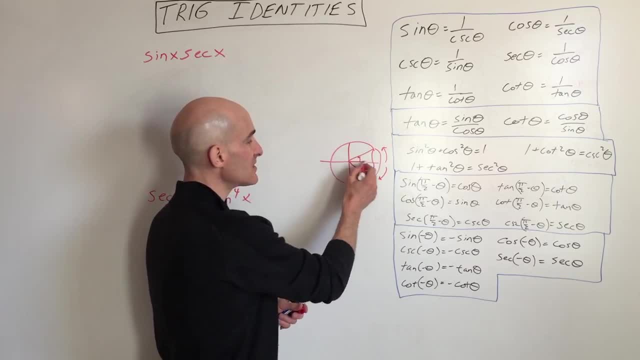 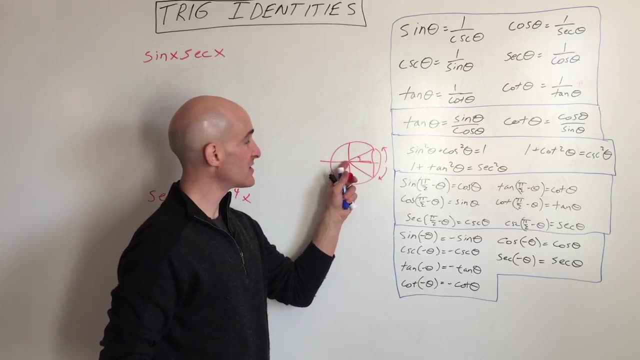 And what you'll notice is: see cosine on the unit circle is the x-coordinate. So whether you go counterclockwise or clockwise, the same number of degrees. these triangles are going to be exactly congruent and the x-value is going to be the same. But notice the y-value. this is positive, this is. 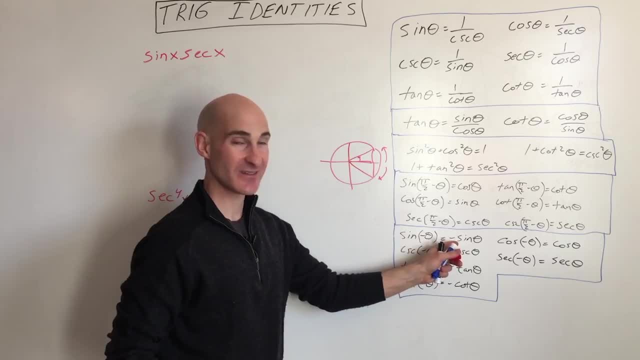 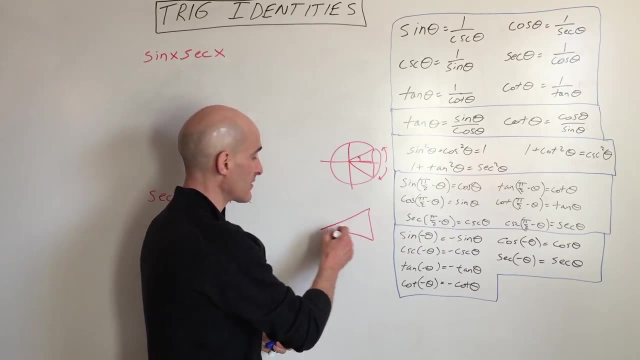 negative And that's why you can see sine of a negative angle is the opposite from the sine of a positive angle, So you can draw diagrams like these. Another one with the co-functions: okay is, if you have a right triangle, and this is theta, this will be 90 minus Thiità. okay, because these 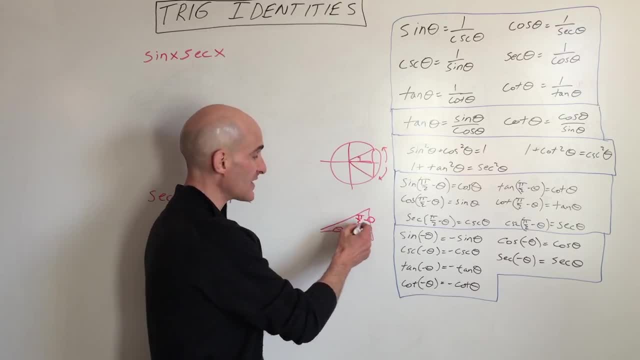 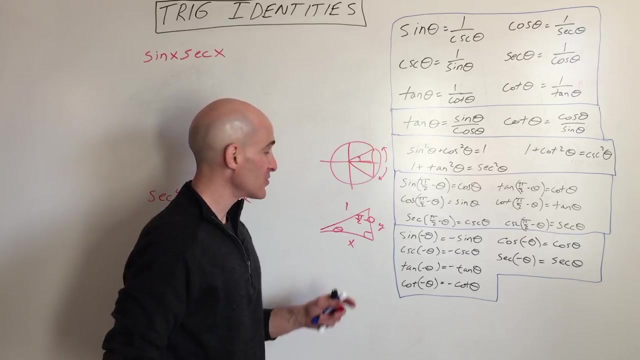 two angles add up to 90. So if you do, the sine sine is opposite over hypotenuse. Cosine of 90 minus angle is adjacent over hypotenuse. But you notice we both uh got y over 1 for both of those. So you can see cosign is adjacent over hypotenuse. Sine of 90 minus theta is: 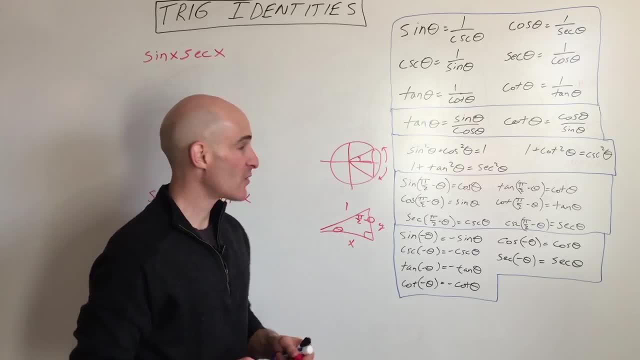 opposite of our hypotenuse, you still get X over one, So that's why they're equivalent. So you can draw some of these triangles to help you understand why these identities are the way that they are. But let's see if we can do some problems, And there's two different types that we're going to. 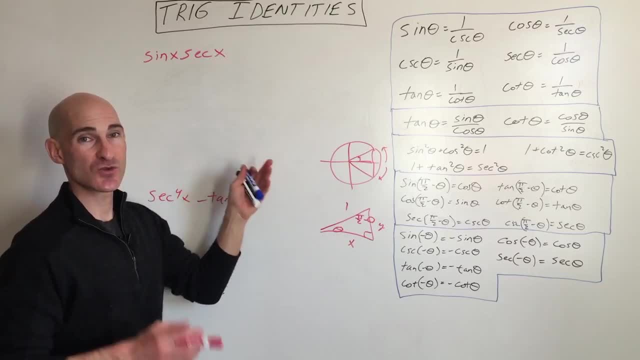 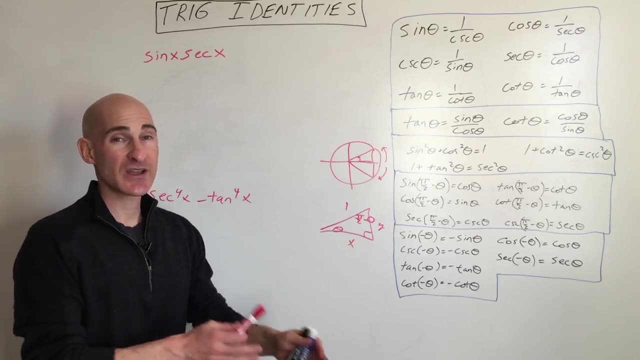 be doing. One is where we're simplifying expressions. We're just trying to condense them down as much as we can. The other type: we're going to be verifying identities. We're going to be basically doing like a trig proof, step-by-step, showing that the left side is 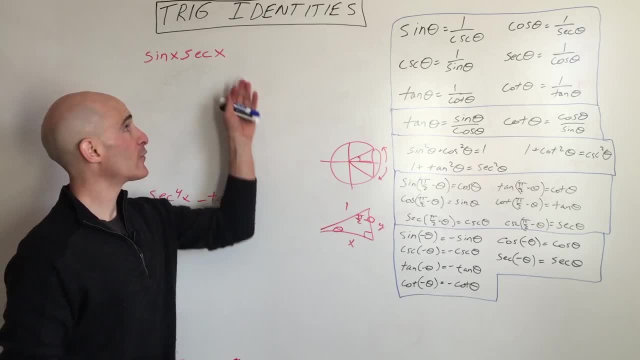 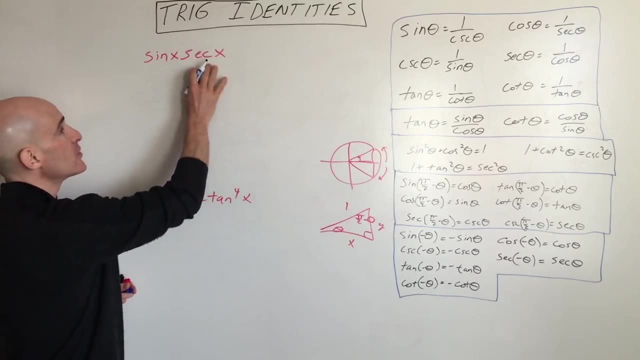 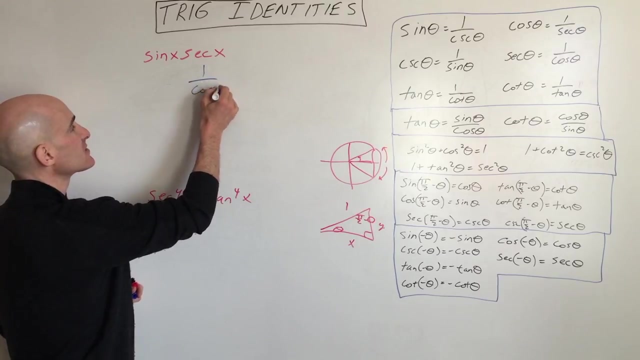 identical to the right side, And so that's called verifying identities. But first let's do some simplifying expressions. So here what we have is sine X times secant X. Okay, so I know, secant of X is one over cosine, So this I could write as one over cosine X. Sine of X is like: 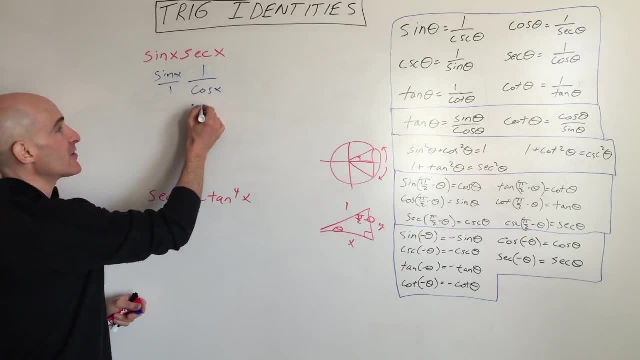 sine over one And if we multiply the numerators and denominators, just like what we learned in algebra and pre-algebra, working with fractions, we can combine And sine over cosine. we know that's tangent. So this is tangent of X And that's about as far as 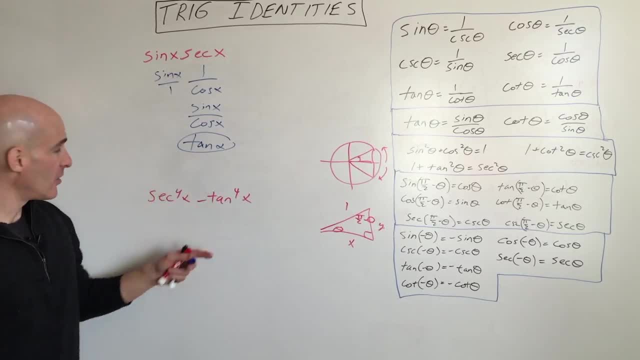 we're going to be able to condense that down. Okay, the next one we've got secant to the fourth of X minus tangent to the fourth of X. What does that condense down to Here? what we're going to do is we're going to do some factoring. So you probably remember from algebra the difference of: 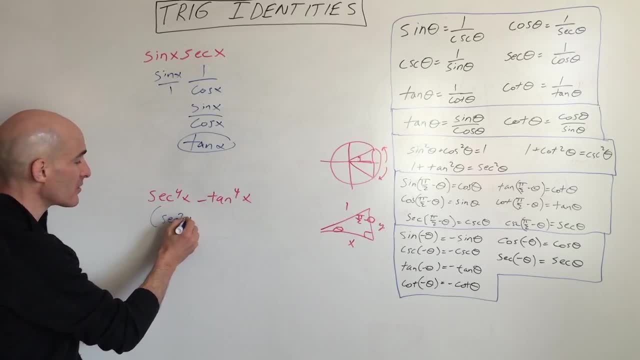 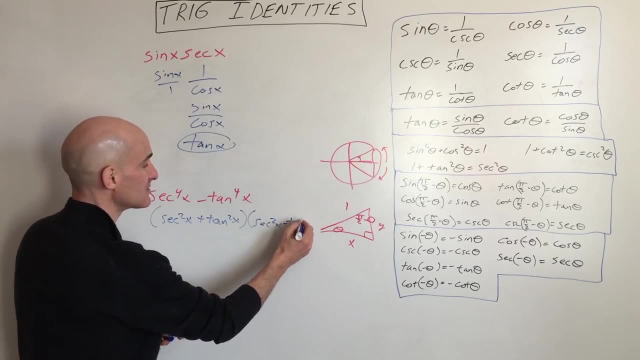 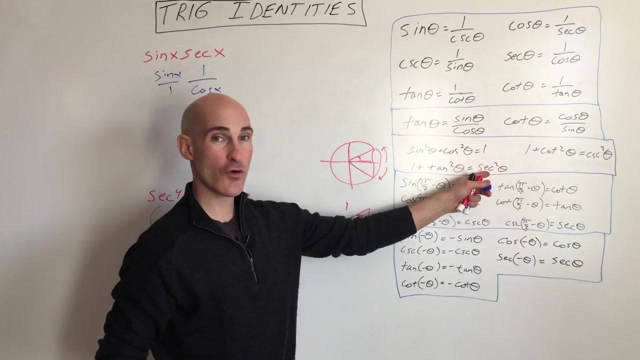 two squares. So that's what we're going to do. We've got secant squared of X plus tangent squared of X Times secant squared of X minus tangent squared of X. Now, what does secant squared minus tangent squared of X equal? Well, you can see if we go over here to the Pythagorean trig identities. 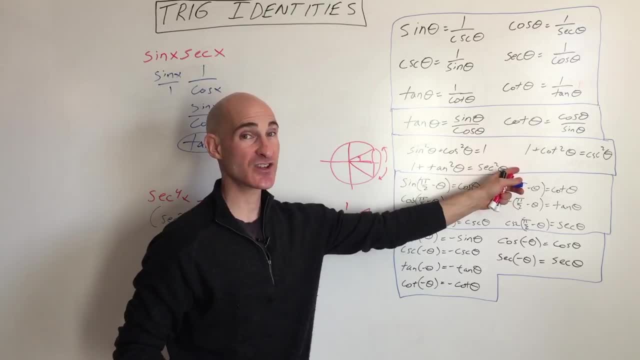 if we subtract tangent squared from both sides of this equation, it's still an identity, It's still the left side is identical to the right side. So we can do that. We'll subtract tangent squared over here. Secant squared minus tangent squared equals one. So this part here is one. 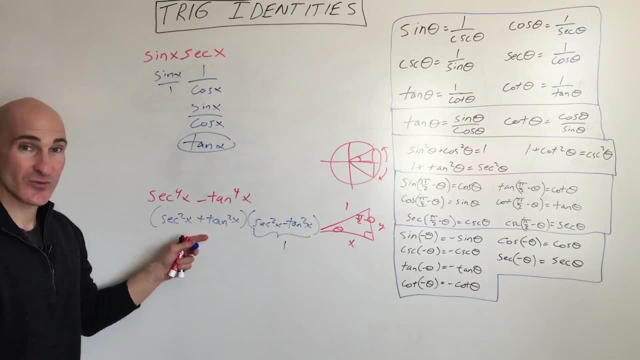 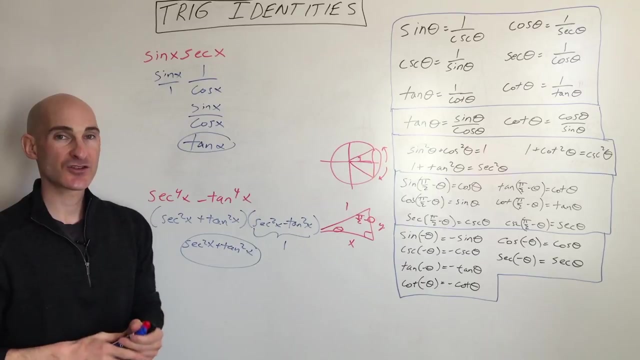 Secant squared plus tangent squared times, one is just going to be itself. So we get secant squared X plus tangent squared X. So that's about as far as we're going to be able to reduce that one now. So here's a couple examples of working with simplifying trigonometric expressions. 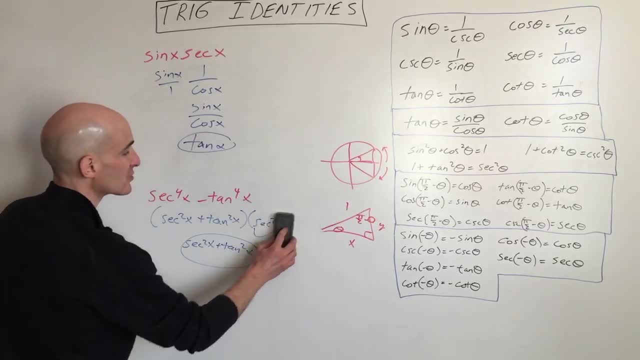 Now let's talk about verifying trigonometric identities. So I'll write down a few problems. When you do these problems, they seem difficult at first, But then you come up with a solution. We go to the next piece here. I'll show you what it is. We look for theрий and then we 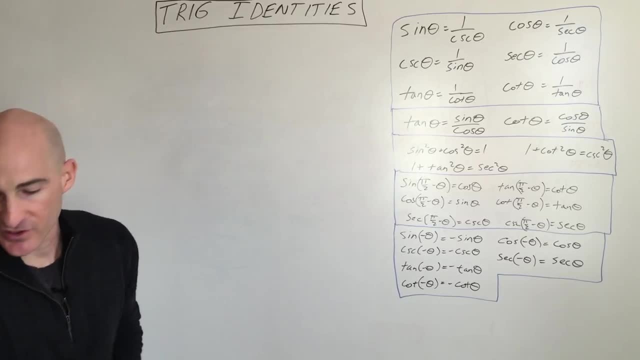 start with they and we look for they, and we look for they, and then we do that again. We go to the next piece here. So if you look at the communities, these three k's, you're going to difficult at first because it's something that you're not used to seeing. but just think of it. 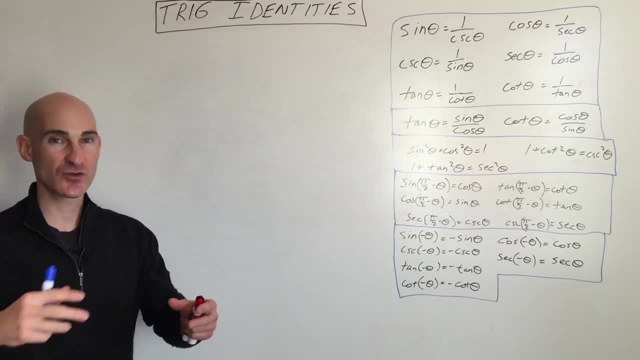 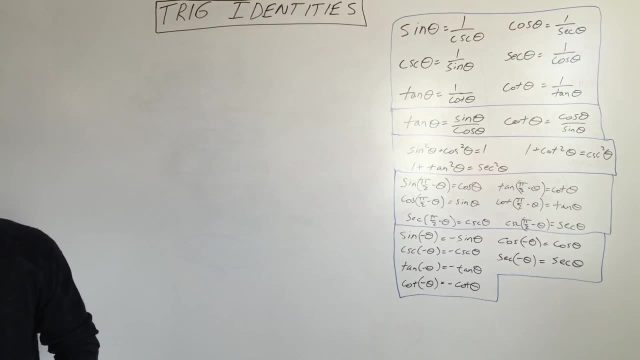 just like algebra, you're going to be doing factoring, you're going to be working with fractions, you're going to be getting common denominators, you're going to be combining, like terms, and so on. so let's do a couple of these ones. let's look at this one here: sine of x. 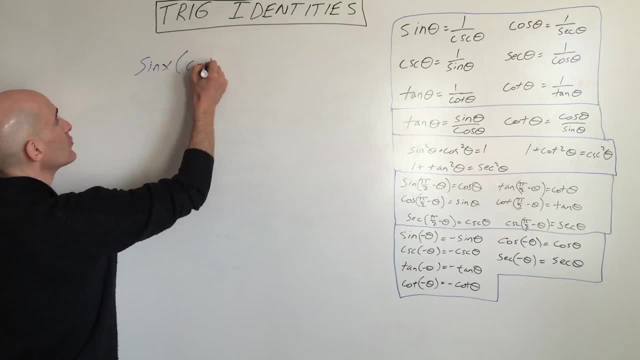 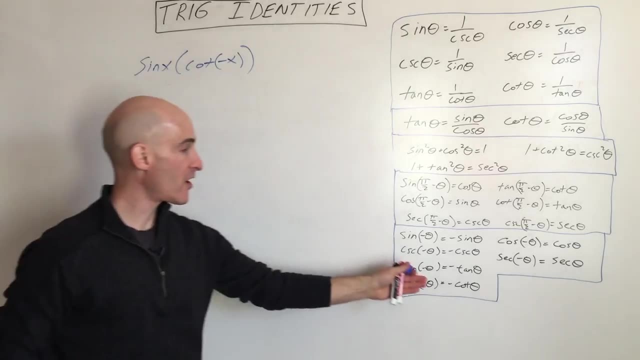 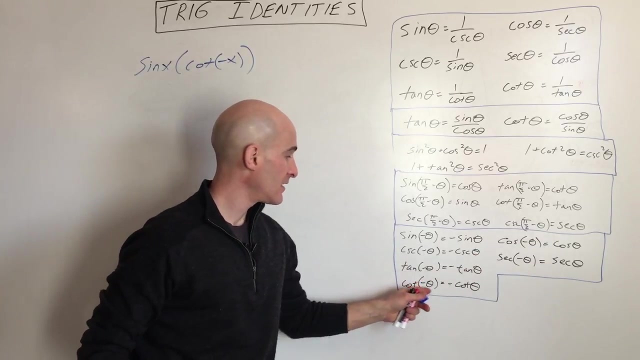 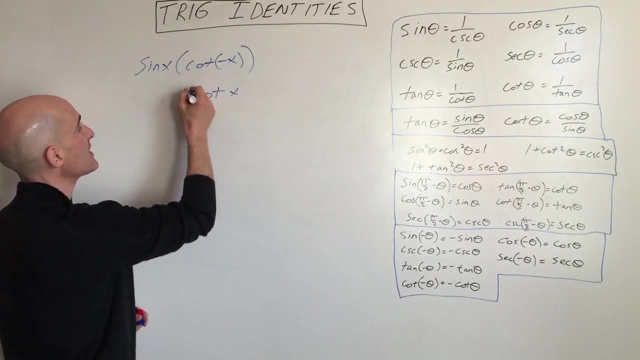 times the cotangent of negative x. okay, so now, look, we've got a negative angle. we go to our even and odd functions. okay, even and odd identities. so cotangent of negative theta is the opposite of cotangent of theta. so let's do a substitution. so this is the same as a negative cotangent of positive x. 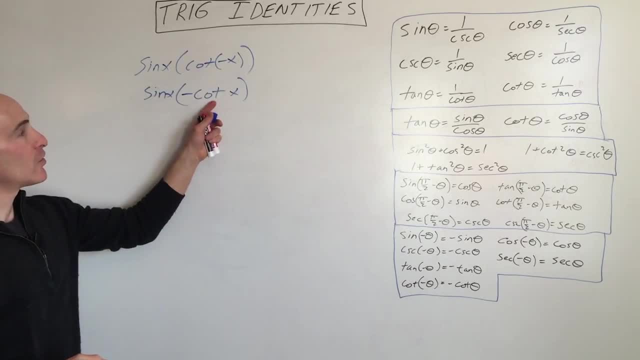 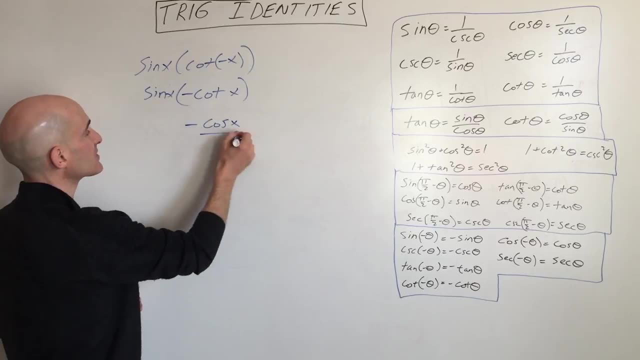 times sine of x. cotangent, we know, is cosine over sine. so this is going to be negative: cosine of x over sine of x times sine of x. that's the sine of x here. okay, you now, when you multiply fractions, remember that you can cross, reduce, right numerator and denominator. 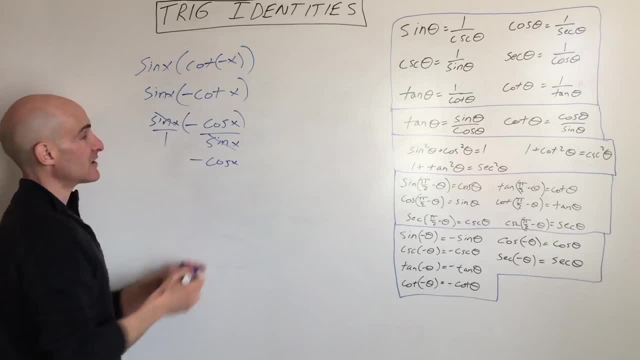 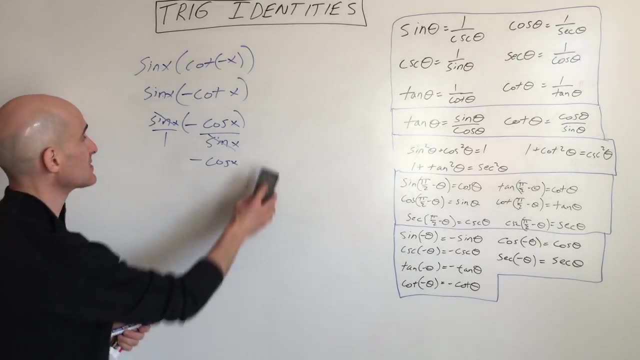 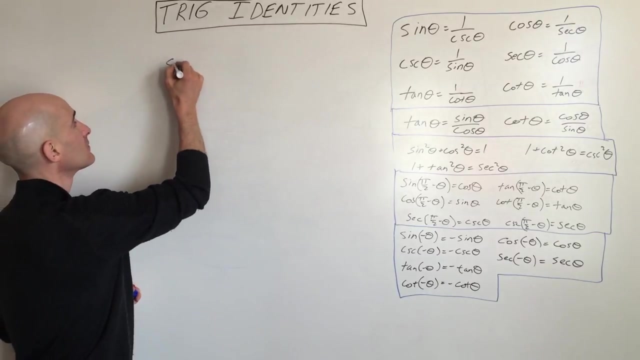 they cancel. so this all reduces down to negative cosine of x. so that was just another simplifying expression. we'll get into the identities. let's do a couple of the verifying identities, okay. so let's take a look at this one here: sine of x times cosecant. 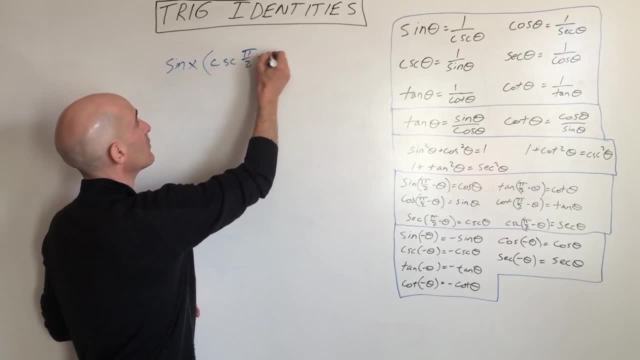 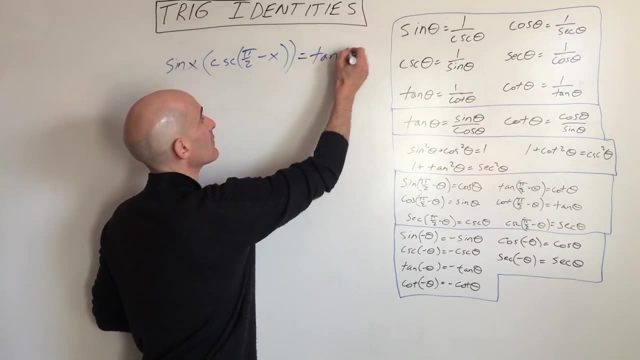 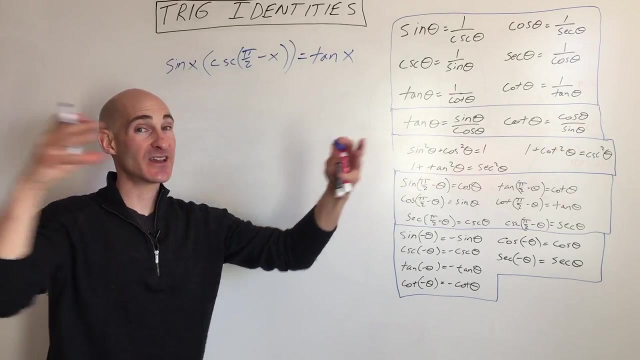 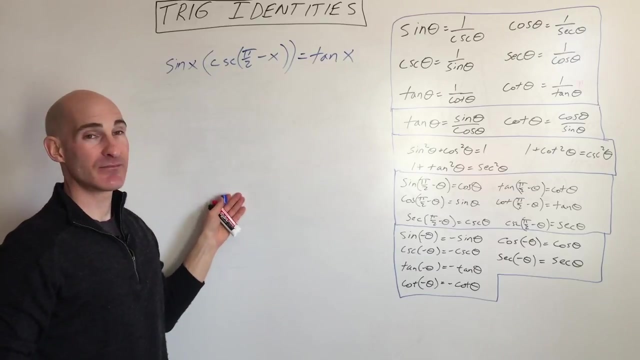 of pi over two minus x equals tangent of x. so when you do these verifying identities, what you want to do is you. you want to work with the more expanded side and you want to condense it to the more condensed or smaller, compact side. usually it's the left side that you're working with and you just step by step. 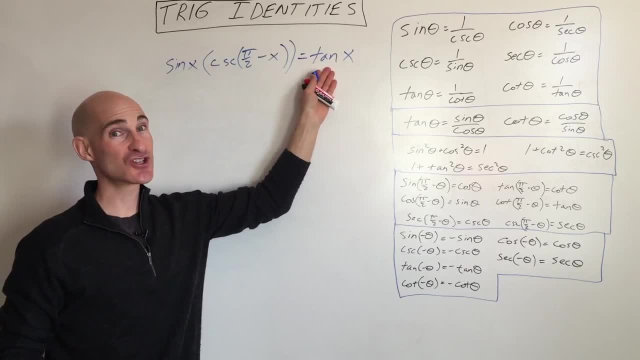 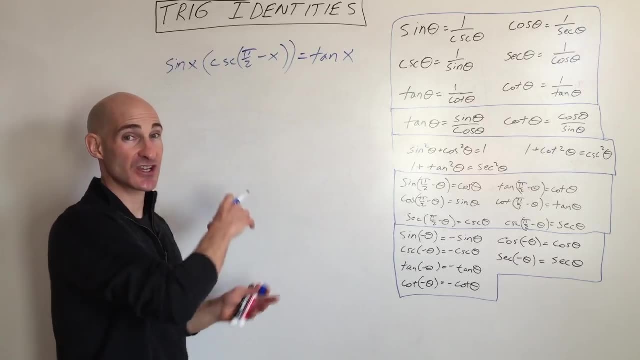 do your substitutions and simplifications until you can show that it equals the right side. but you could flip it. you could start with the right side, step by step, show the substitutions and simplifications and show that equals the left side. but you don't want to be moving anything from left side to right side, like that. 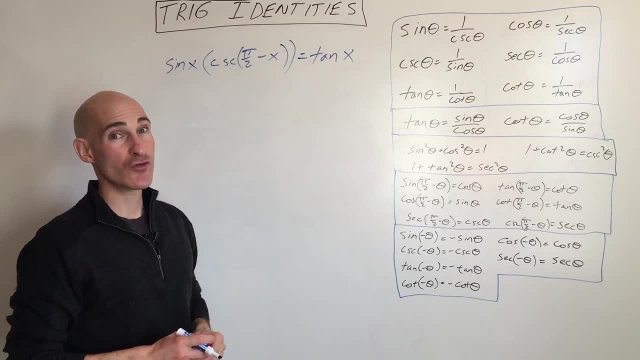 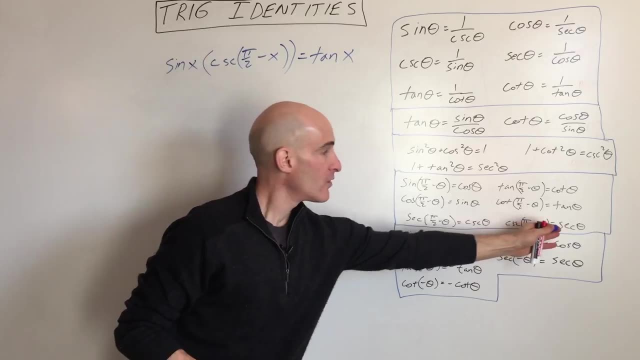 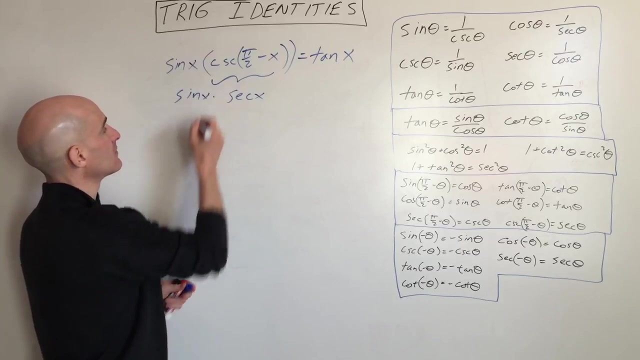 it's not solving an equation, it's just doing like a trig proof and verifying one side equals the other. so cosecant of 90 minus x- we're going to go over to our cofunctions here- equals sequent of x. so this here is secant of x times sine of x. 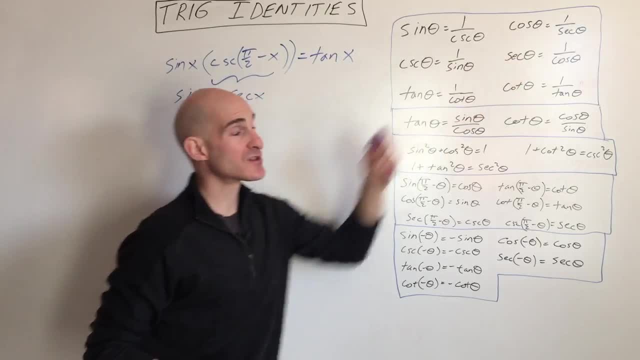 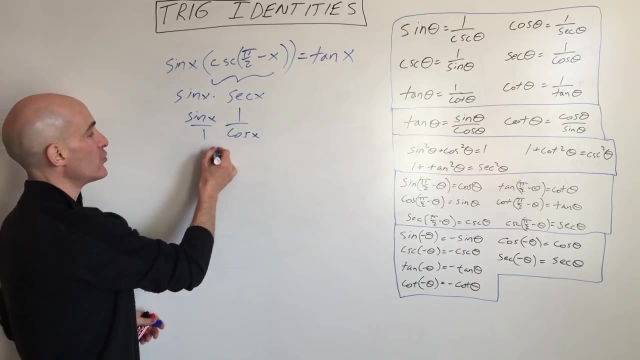 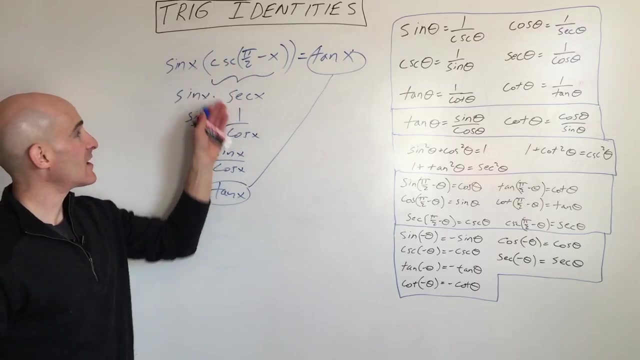 secant of is equal to 1 over cosine, so this is 1 over cosine. you can multiply the numerators and denominators: sine over cosine equals tangent. so this is tangent of X. and you can see they're identical. so we proved it step by step. you don't. 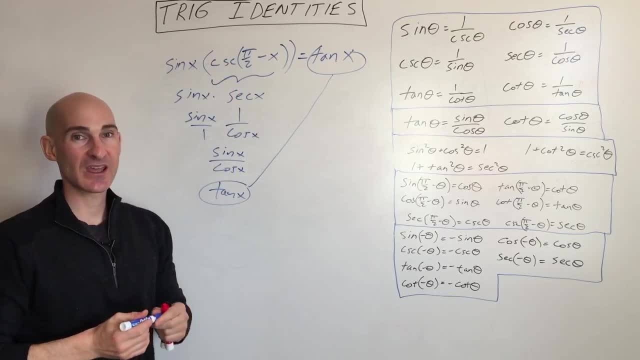 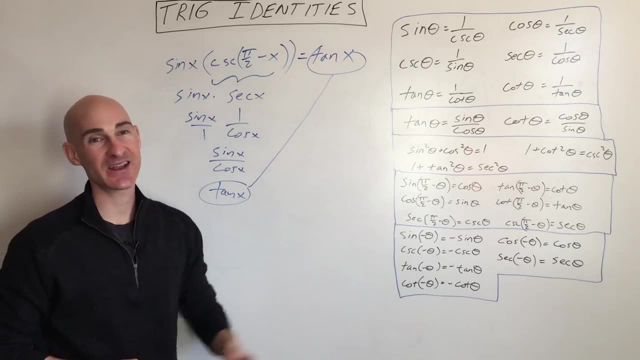 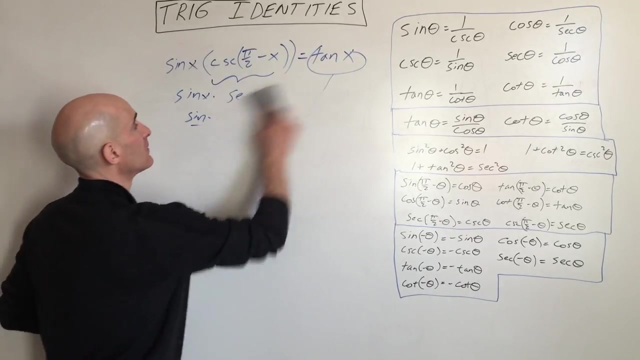 want to skip too many steps. you want to show what substitutions you're making in and simplifying, and you can even go so far as to say, like I used a reciprocal identity, or I used a co-function, or I use an, even an odd identity to justify your step. let's do another example. sometimes, when you're 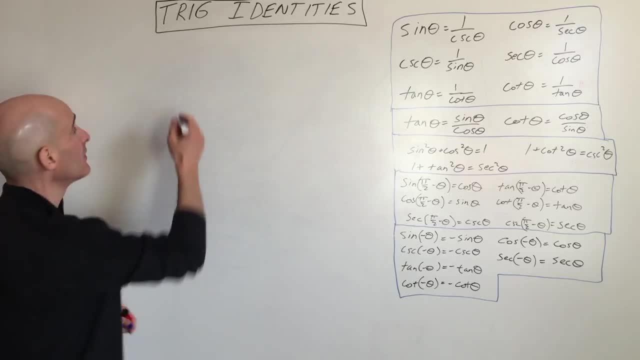 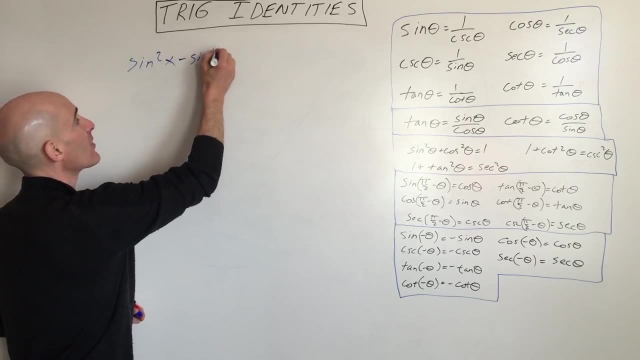 doing these problems, students get stuck and they just say: I don't know what to do. so you know, I'm just gonna stop. and even if you don't know what to do, one of my math professors always just said: do something. just do something, because sometimes you take that first step and that'll lead to something else and 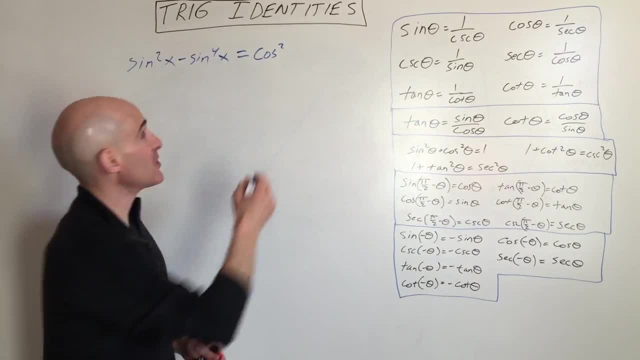 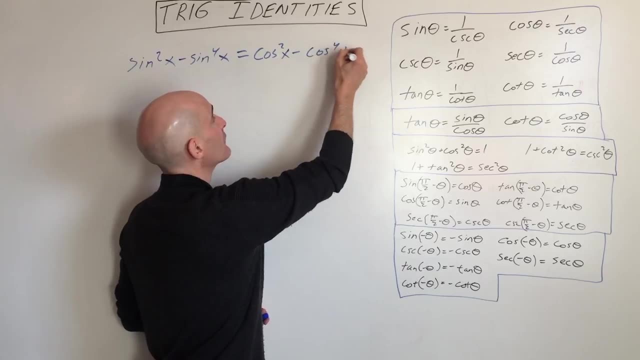 something else and something else, and before you know it, you solved it. but you have to take that first step, even though you don't necessarily know what the next step after that's going to be. just take that first step and if you make a mistake, of course you know you're going to learn something even from that. 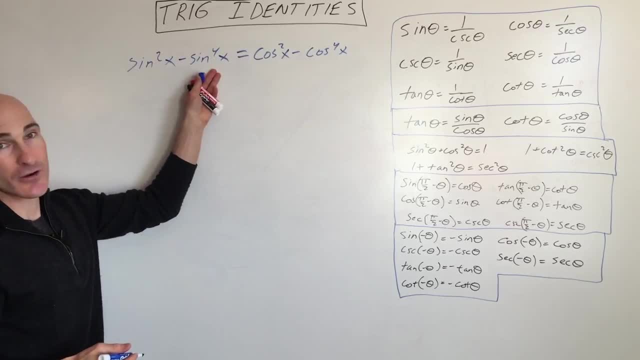 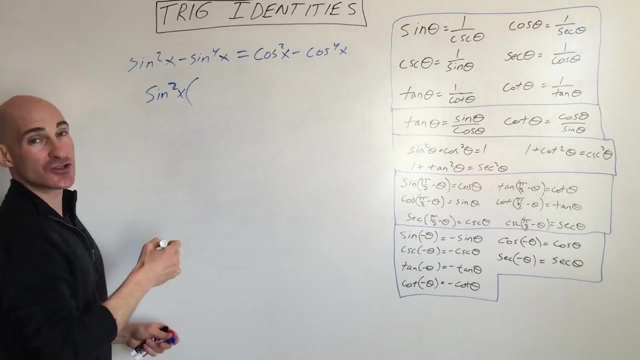 mistake. so let's take a look over at this side here. okay, we're gonna try to show that this side equals this side. okay, we can divide out a sine squared, so that's using the greatest common factor factoring technique we learned in algebra. right, so that's going to be 1. 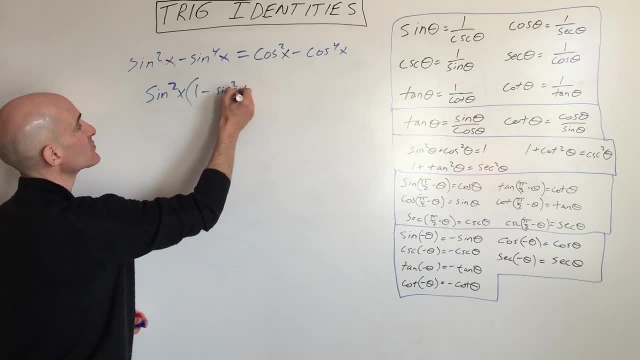 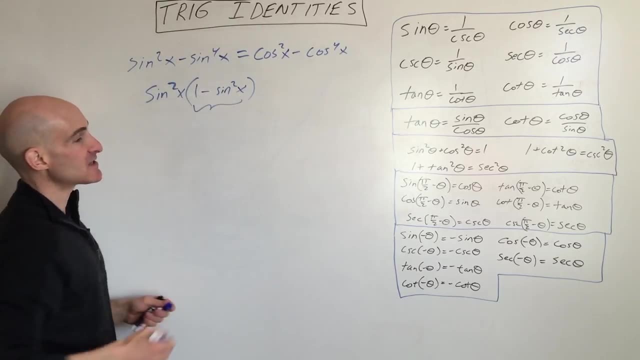 minus sine squared of X. so I just factor out a sine squared. so we're just doing algebra, but with trig functions. and then now we have 1 minus sine squared. hmm, let's see 1 minus sine squared if I subtract sine squared from both sides of. 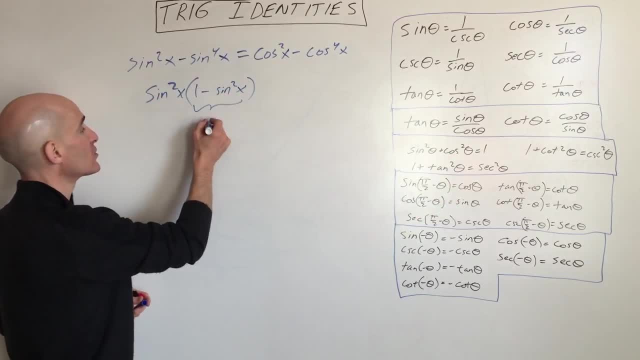 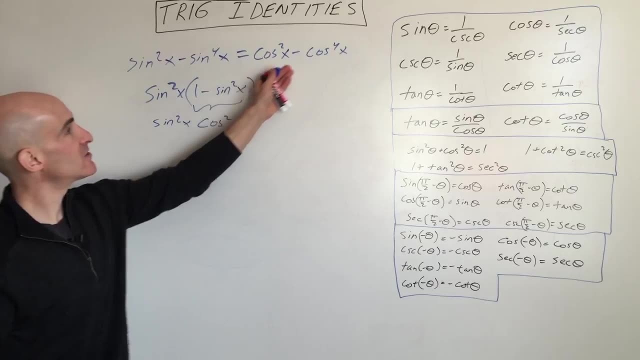 the equation that leaves us with cosine squared. okay, so we're going to do that cosine squared. Okay, so we're going to do that substitution cosine squared of x. okay, times sine squared of x. Hmm, still doesn't look like that, but I noticed. these are all. 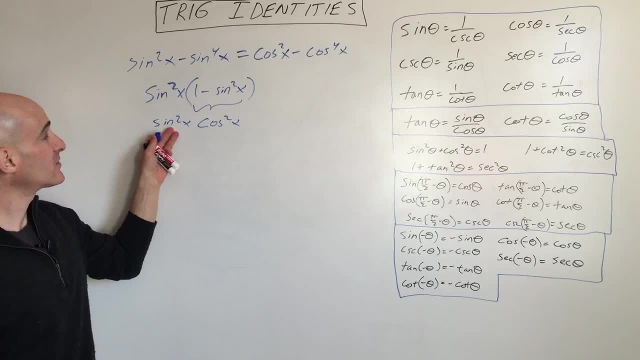 cosines. I have a sine here. still, What does sine squared equal? Sine squared equals one minus cosine squared. So let's do that. Let's replace this with one minus cosine squared, Okay, and we're going to do our distributive property just like we learned in Algebra 1,. 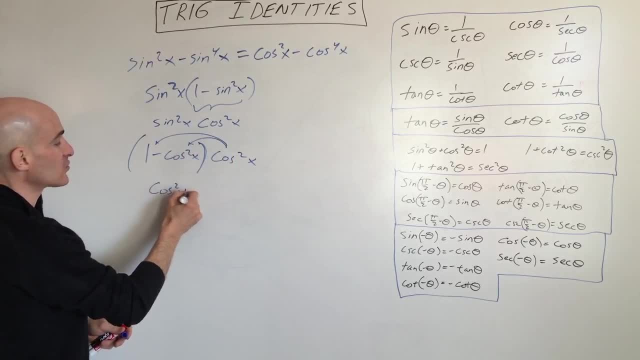 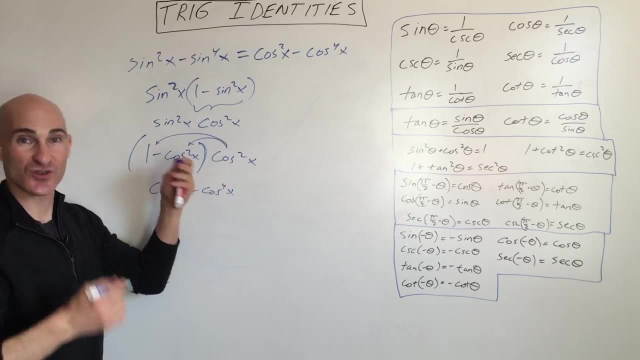 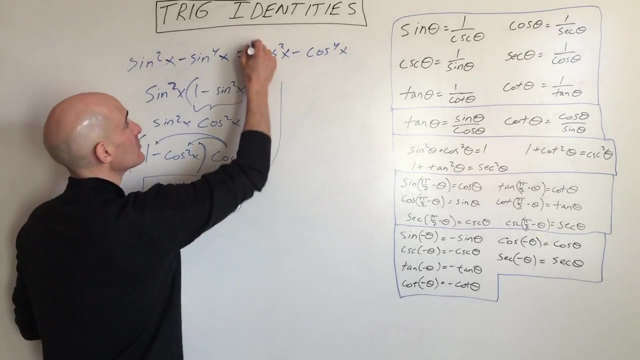 right. So we distribute, and what do we get? Cosine squared x minus cosine to the fourth x. Remember, when you multiply you add exponents if you have the same base. So it's just algebra You can see, just with trigonometric functions. And so there we go. The left side equals the right side. 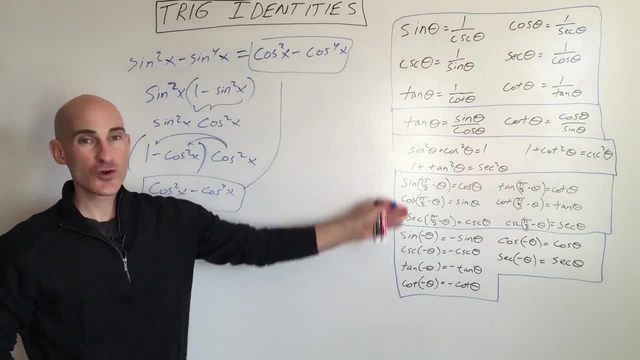 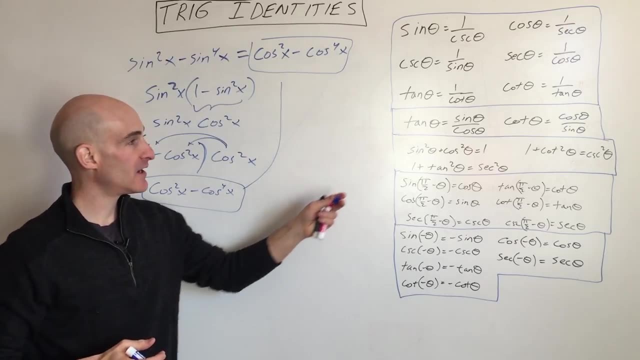 and we proved it. So get familiar. Get familiar with the identities. It helps if you memorize them, because when you're doing these problems they tend to jump off the page a little bit. You say, oh, that looks a lot like this one.